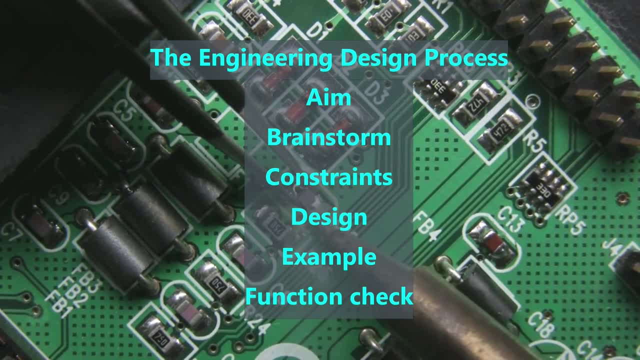 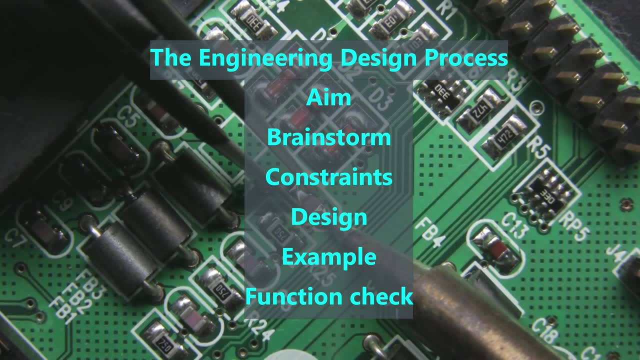 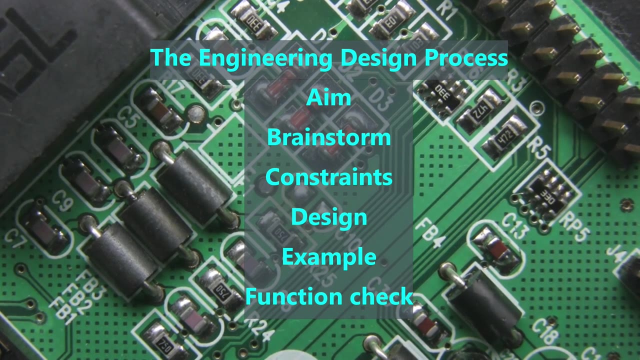 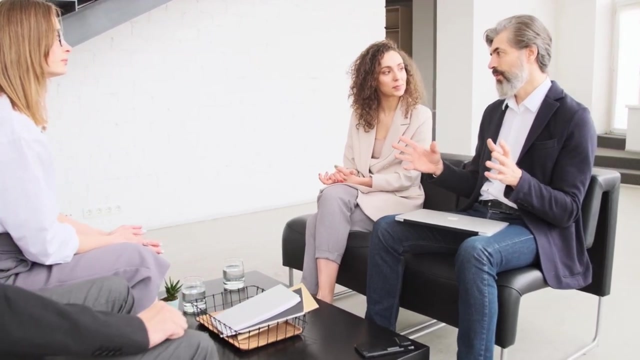 We chose these words so that the names of each step and the order it comes in is easy to remember with the acronym ABCDEF. The steps are: aim, brainstorm, constraints, design, example, function check. Before we show engineering scenarios, let's start by applying the engineering design process. 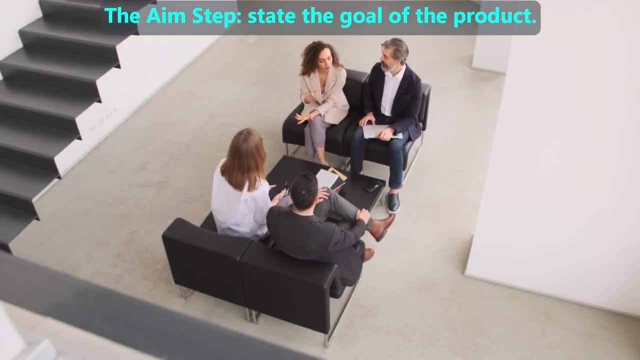 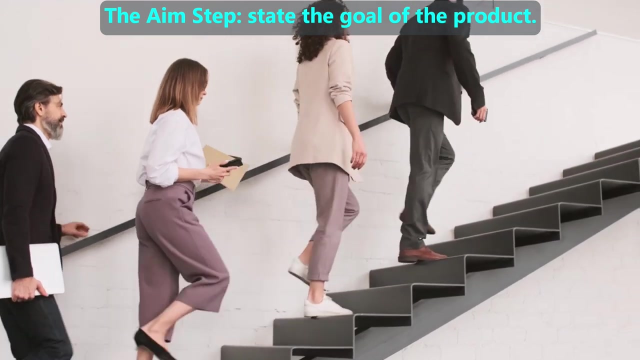 to a cooking scenario. Susie and her office colleagues are planning a small lunch party for the new employees in their office. The lunch will be tomorrow. Susie volunteers to make the dessert and the manager gives her $20 for ingredients. The first step in the engineering design process is to set the aim, which we sometimes call. 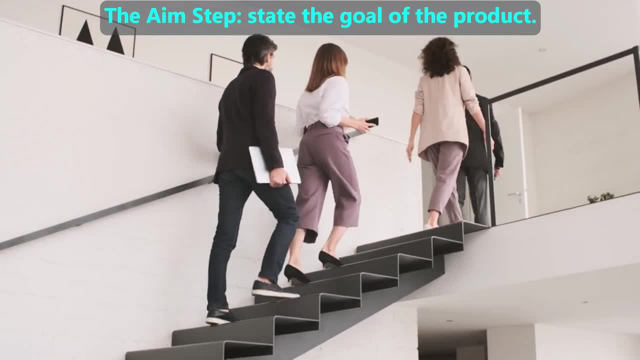 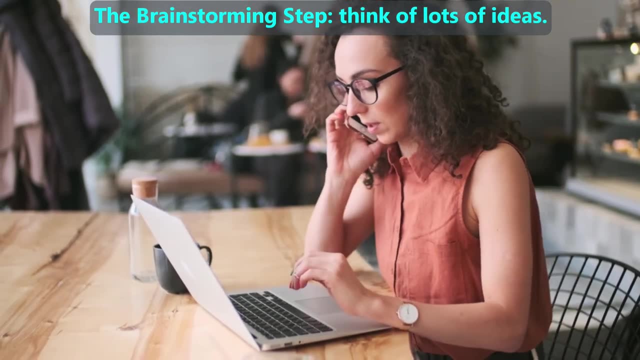 the goal Susie sets her aim to be that the dessert is so delicious that almost all of it is eaten. The second step in the engineering design process is to brainstorm. Susie is a good cook, so she wants to make a new recipe. 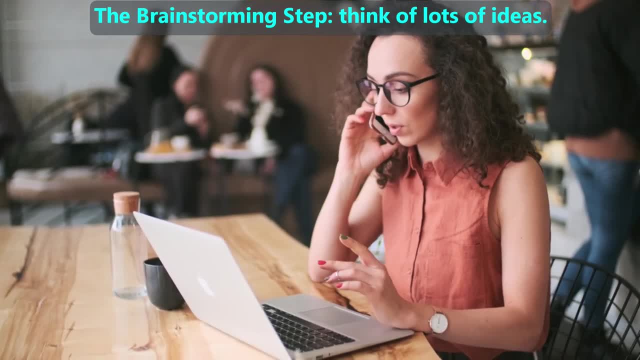 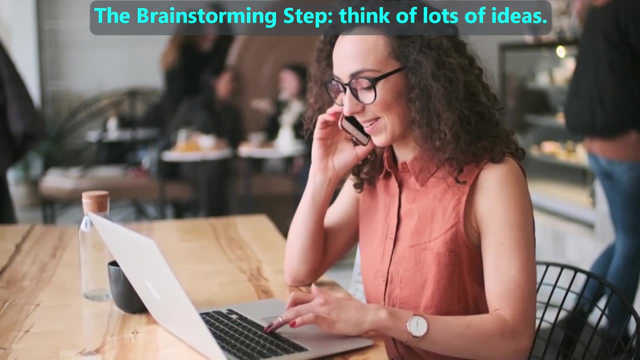 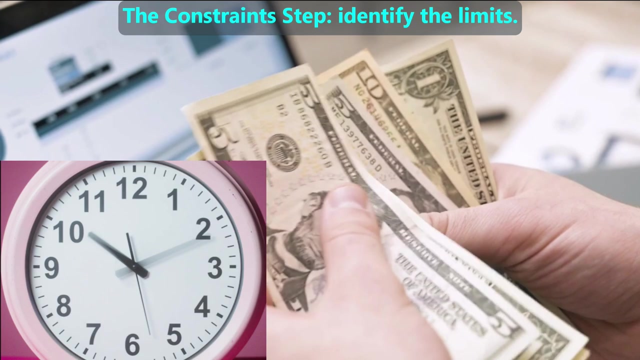 She thinks of a few ideas, but she also calls her family and friends to get their ideas too. She writes down every possible idea, even the ones that seem a little silly at first. The third step in the engineering design process is to identify the constraints. 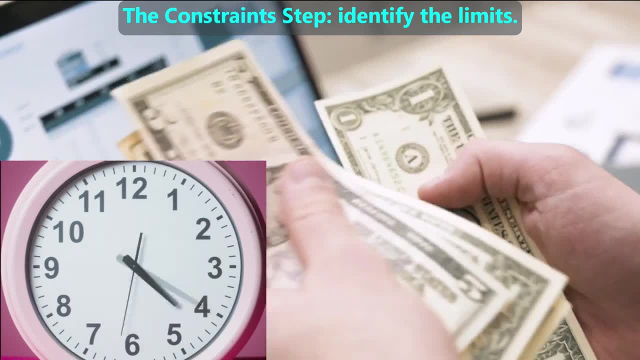 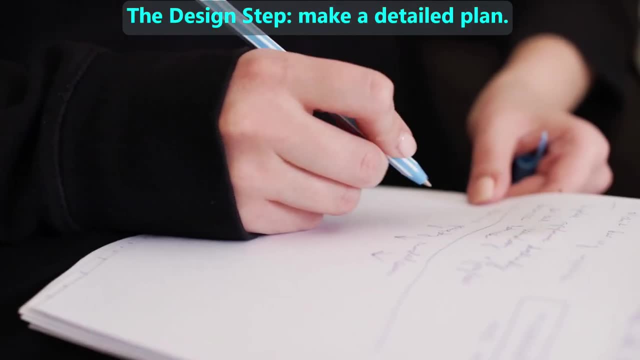 We can think of constraints like limits. The lunch party is tomorrow. She also has to stay within a $20 budget. The fourth step in the engineering design process is to identify the constraints. We can think of constraints like limits. The fourth step in the engineering design process is to design the product or process. 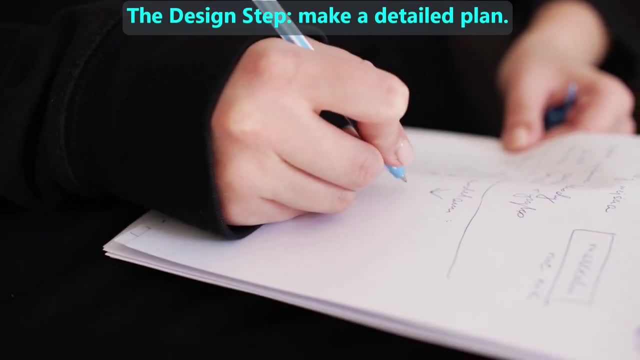 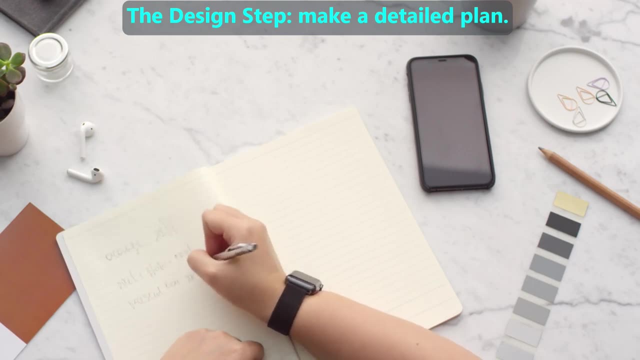 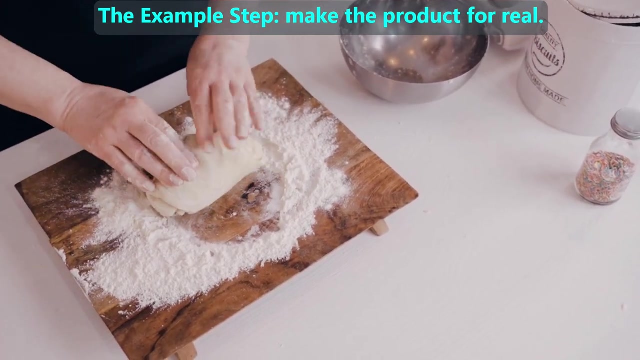 Susie picks a dessert idea that she got during the brainstorming step that will stay within the constraints. She then writes out a detailed recipe with all the ingredients, how much of each to use and how to prepare them. The fifth step in the engineering design process is to make an example product. 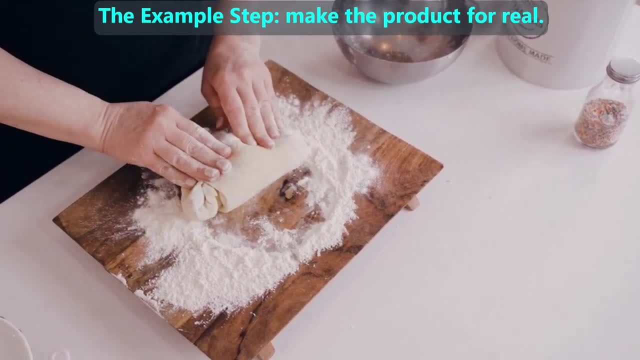 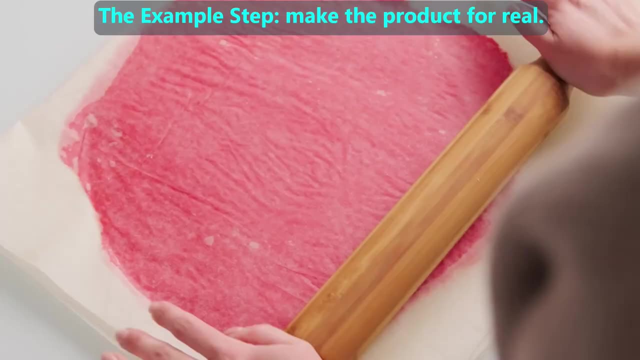 We call it an example because this may not be the final product. We call it an example because this may not be the final product, but rather it is a test one. Engineers often call the example product a prototype. There are usually a lot of prototypes before they settle on a final product, which may 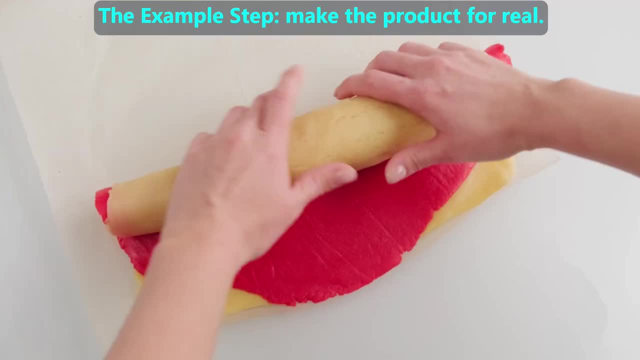 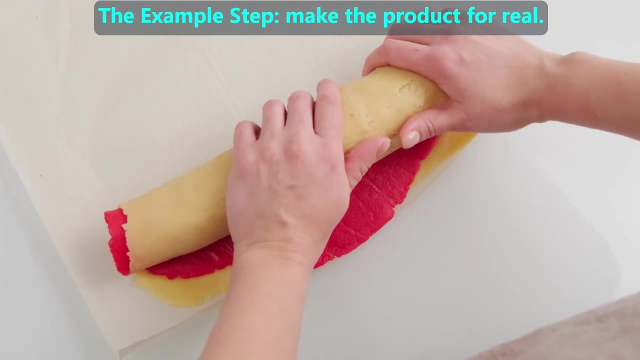 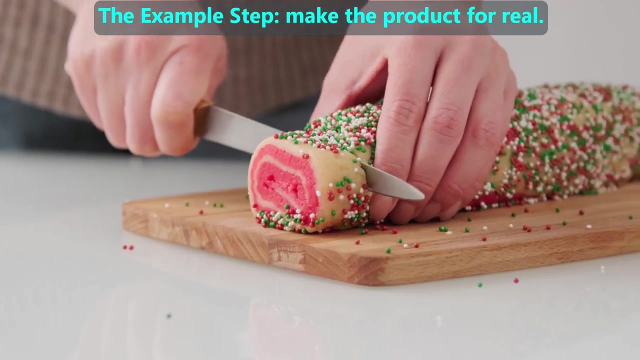 go into a factory where millions will be made. In the example product step, Susie is making the dessert according to the design she made in the prior step. She is following the recipe that she planned in the design step. Susie is using real ingredients and in real portion sizes. 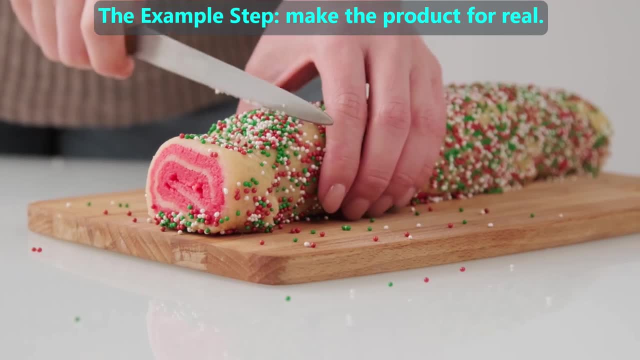 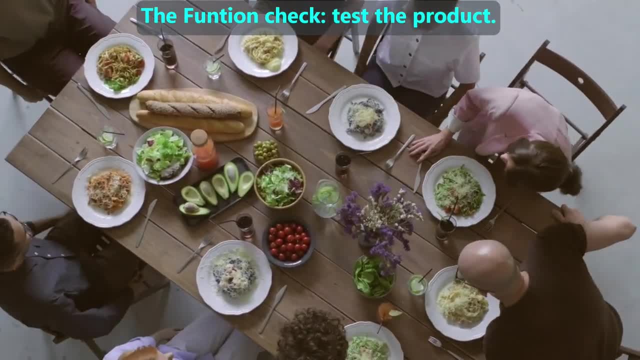 The sixth step in the engineering design process is a function check. The sixth step in the engineering design process is a function check. Sometimes we call this a test. Sometimes we call this a test. The sixth step in the engineering design process is a function check. 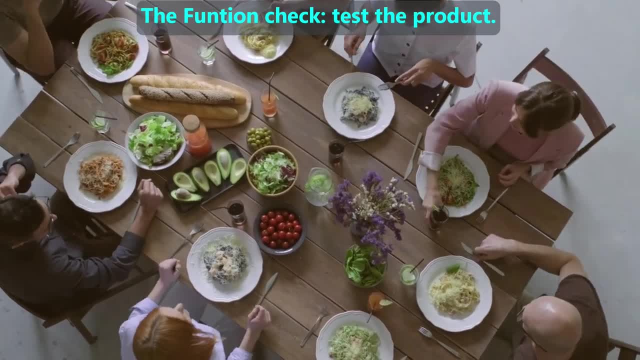 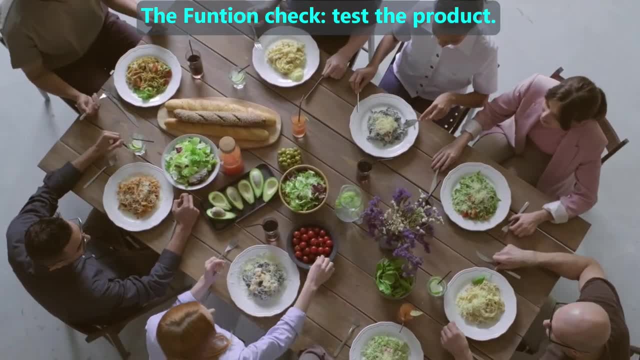 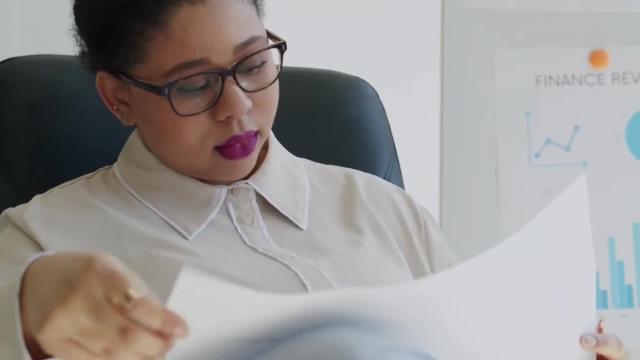 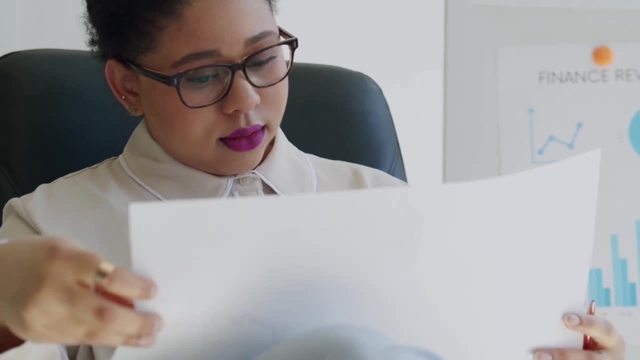 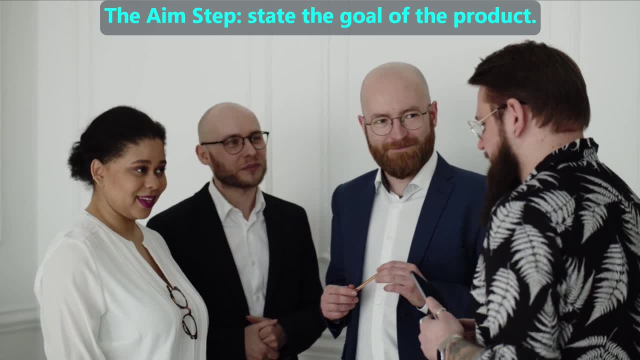 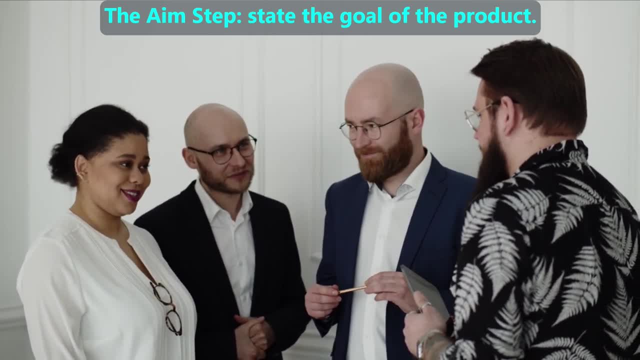 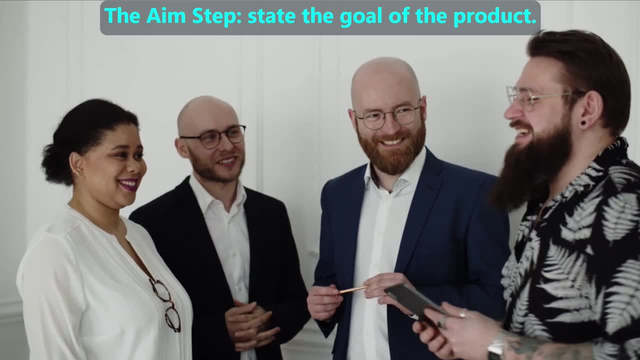 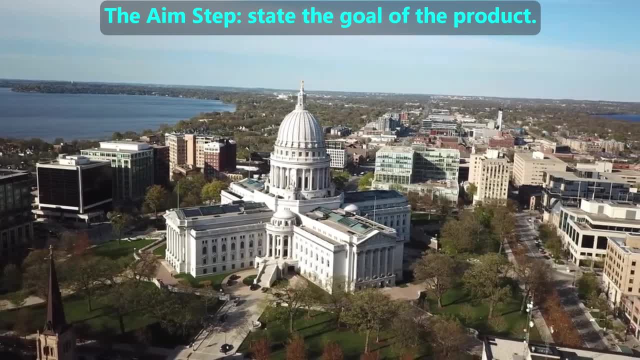 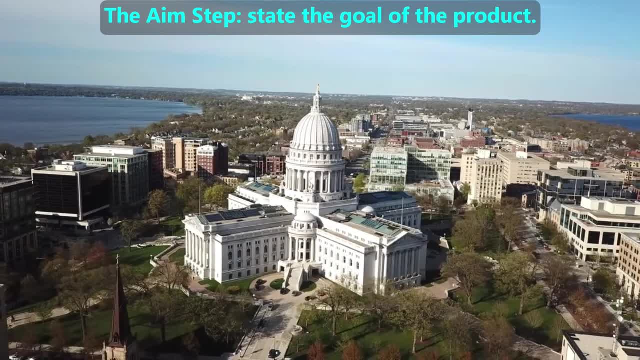 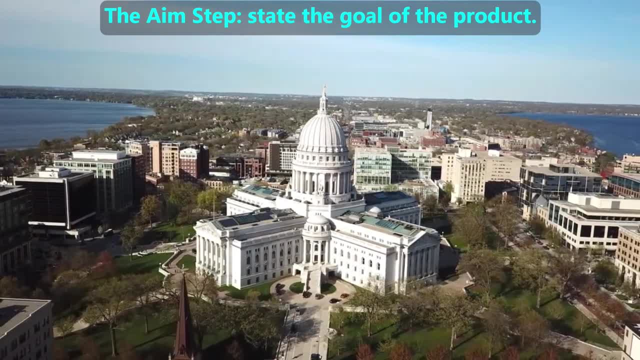 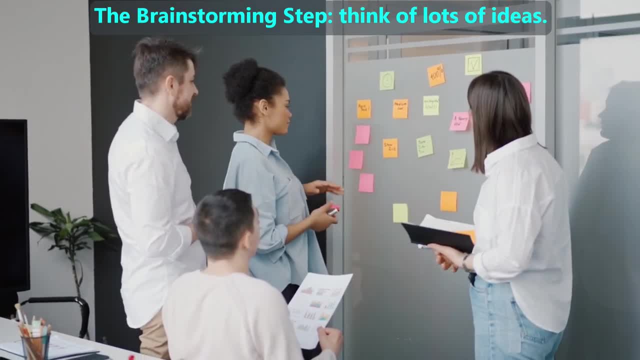 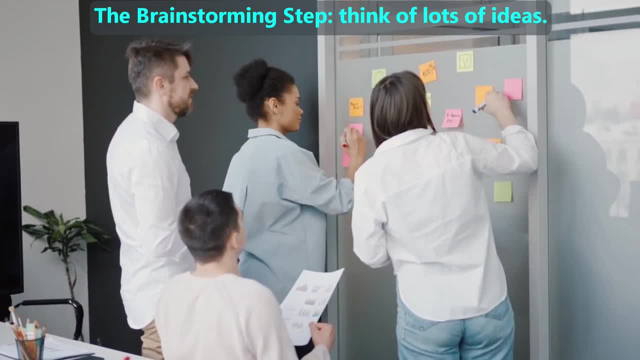 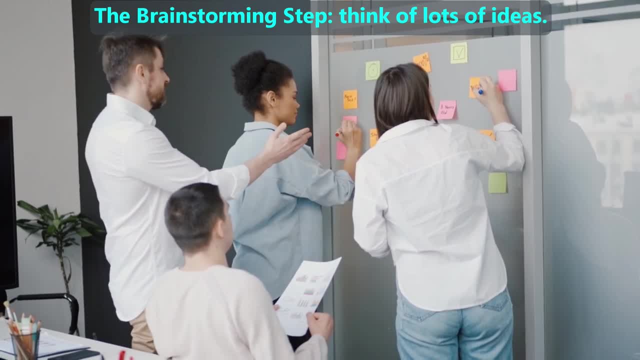 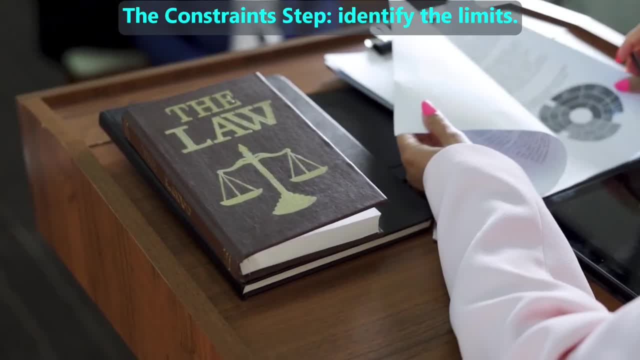 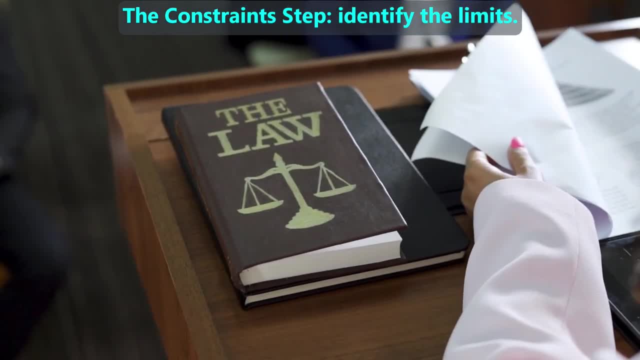 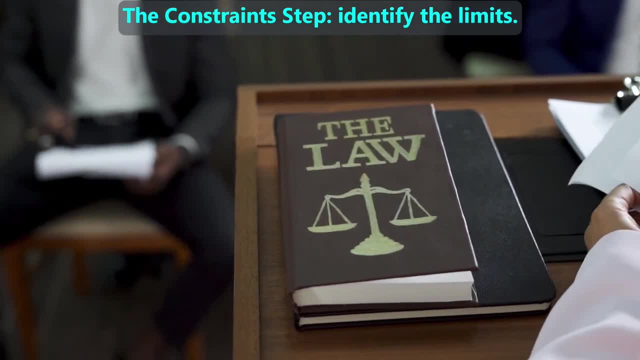 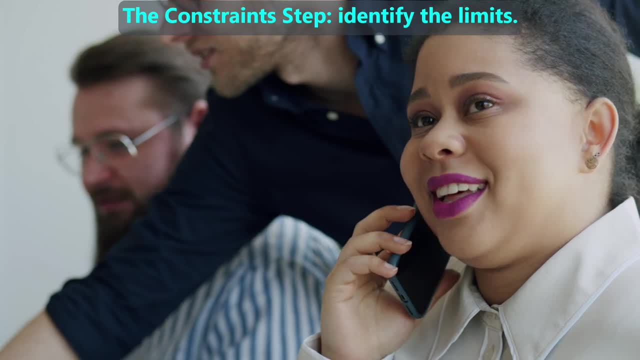 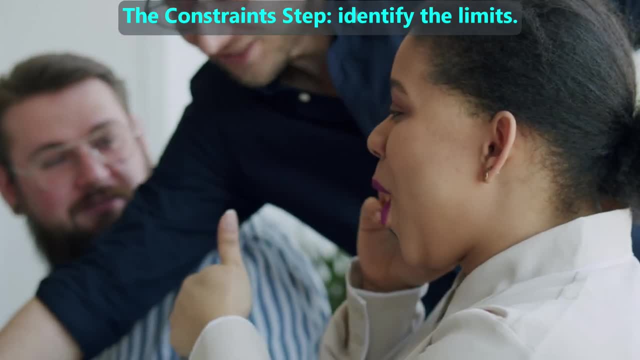 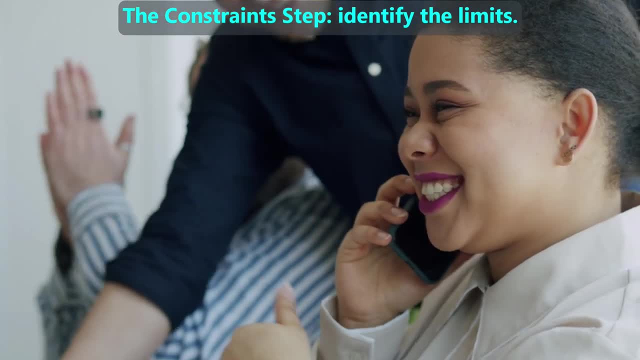 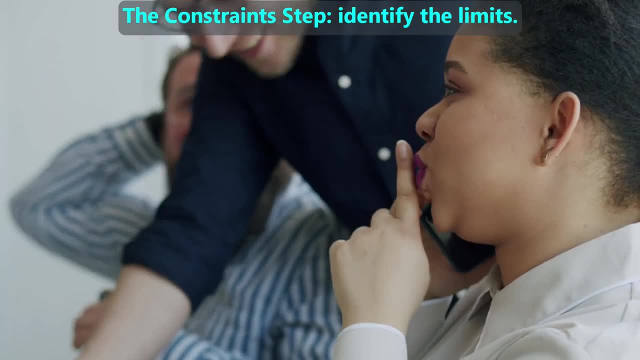 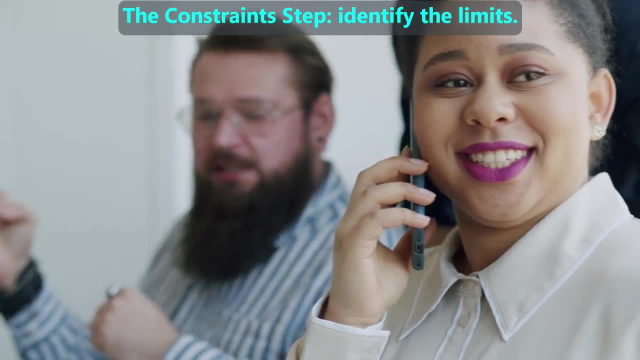 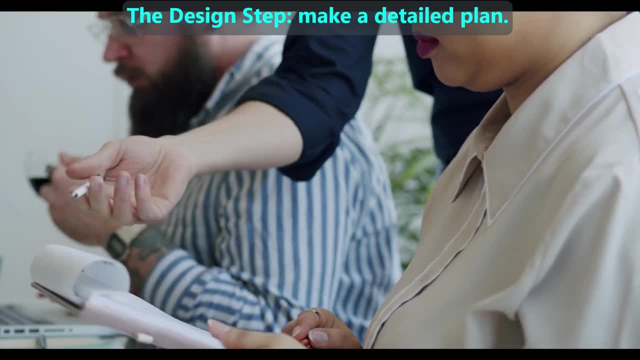 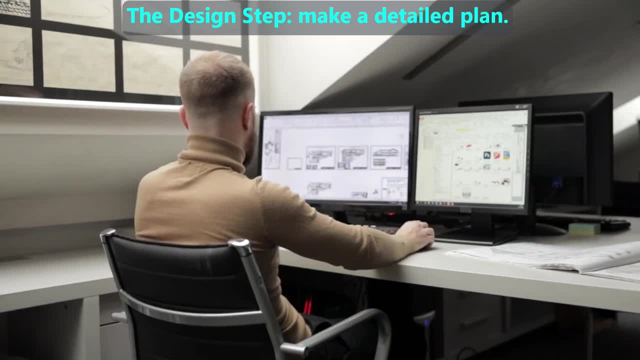 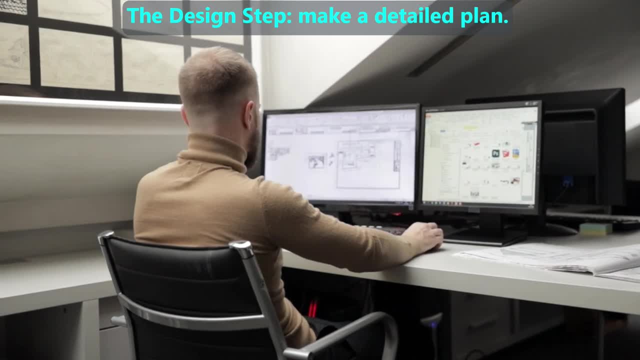 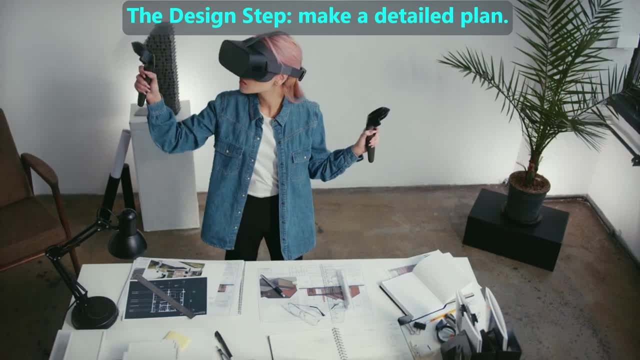 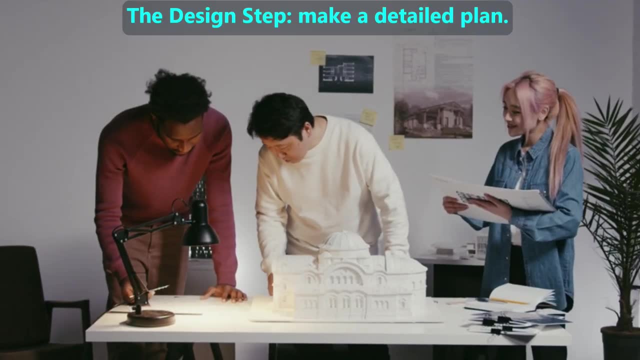 The sixth step in the engineering design process is a function, check detailed blueprints on computers and then make a virtual reality simulation so the user can feel like she or he is inside the museum. They also make a 3D printed model of the museum. 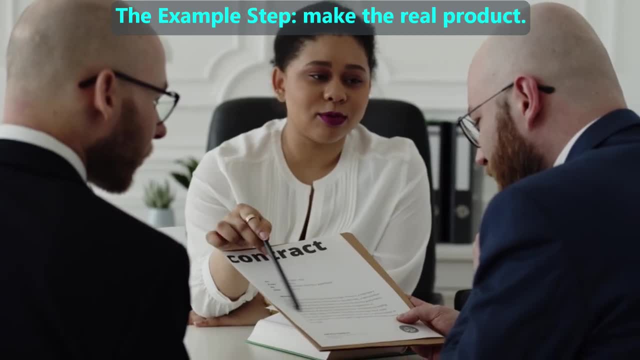 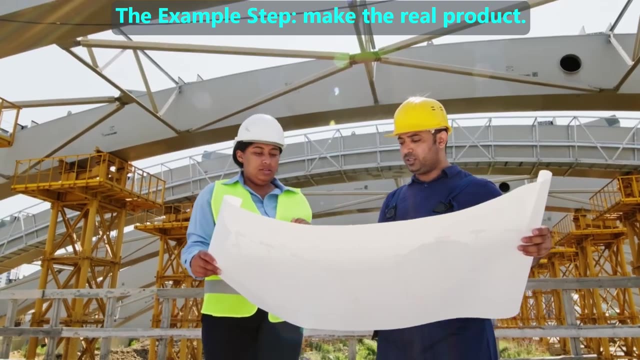 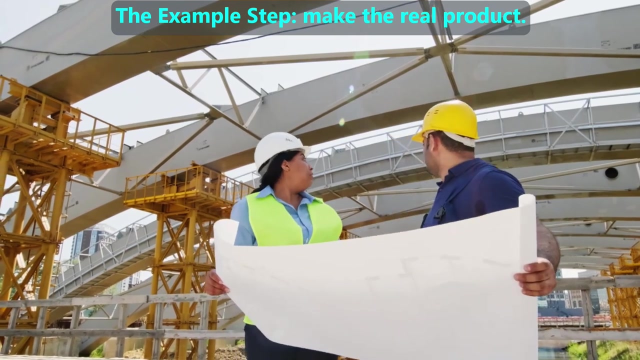 This is the design step. The artists approve the design. so now Angie's team works with contractors to make the building. They are using real materials and it is in the real size. We call this the example step, but for one-of-a-kind projects like this, this is the final product. 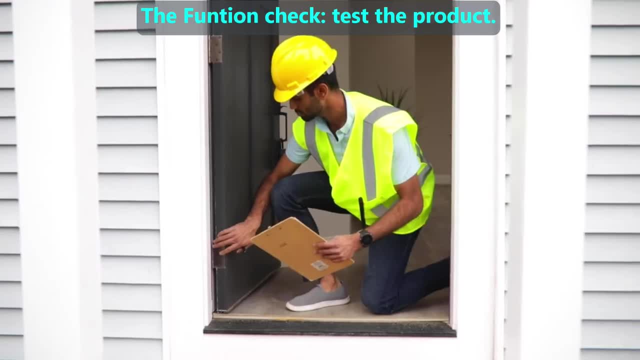 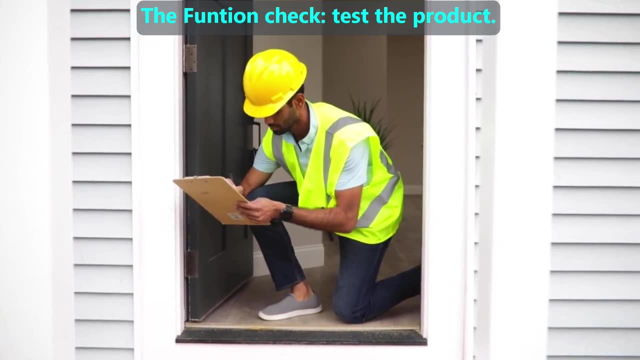 and not an example product like a prototype. The final step of the engineering process is to do function checks. Angie's team has to make sure the building meets the aims the clients gave them. If it doesn't pass a function check, then she makes minor design changes and builds. 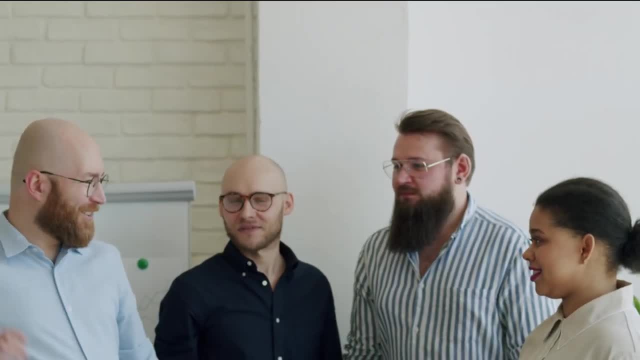 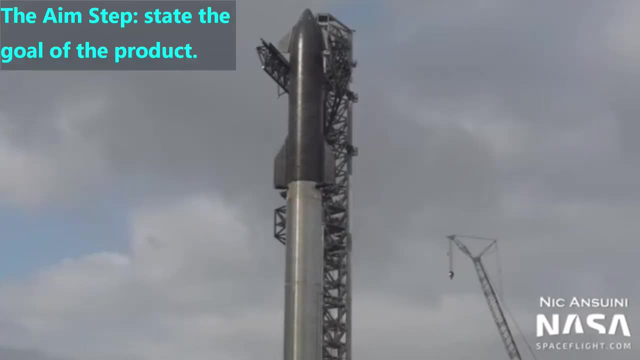 a part slightly differently. In this case, the clients are very happy with the final product, which is a new art museum. For the second scenario, let's imagine how SpaceX engineers develop the top part of this rocket, which is called Starship. 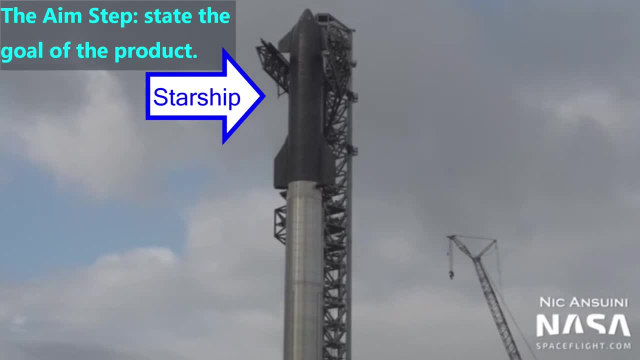 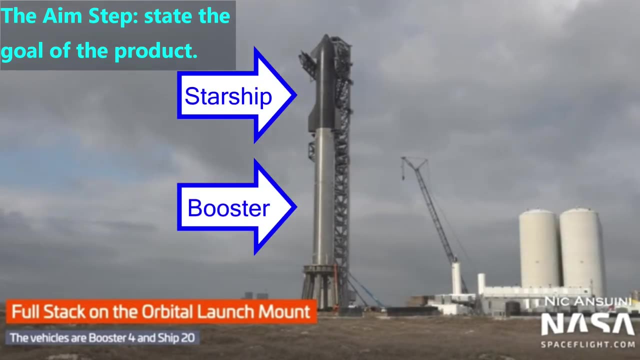 Their aim was to have Starship be able to land after it is launched as part of this huge rocket. The bottom part of this rocket is called a booster and will lift Starship many miles above the ground. then Starship and the booster will separate and the aim is to have both. 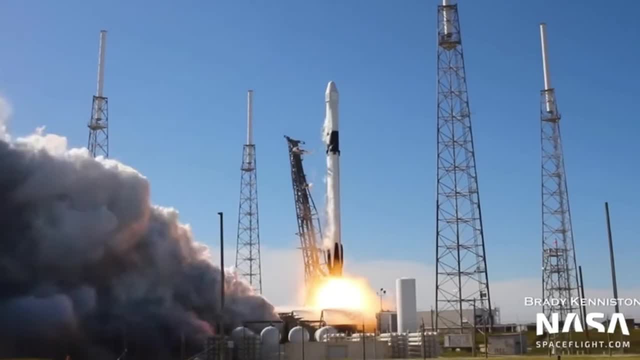 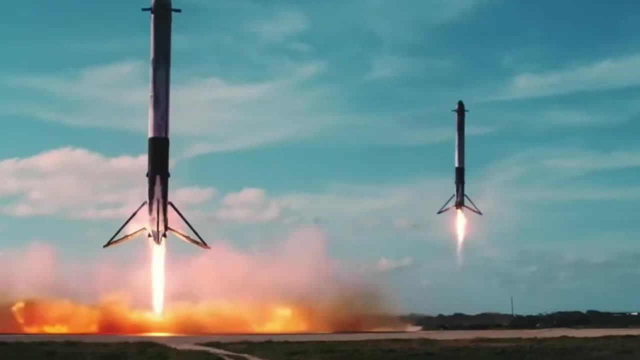 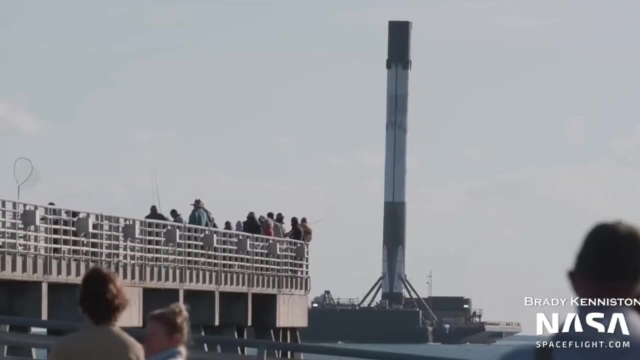 of them land at different times. SpaceX has already figured out how to have smaller boosters land on the ground and they have launched the top part of other rockets. SpaceX has been able to get smaller boosters to touch down on the land And on drone ships. then those ships bring the boosters back so they can be reused. 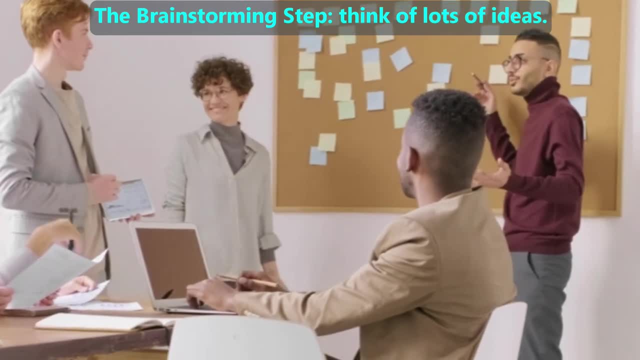 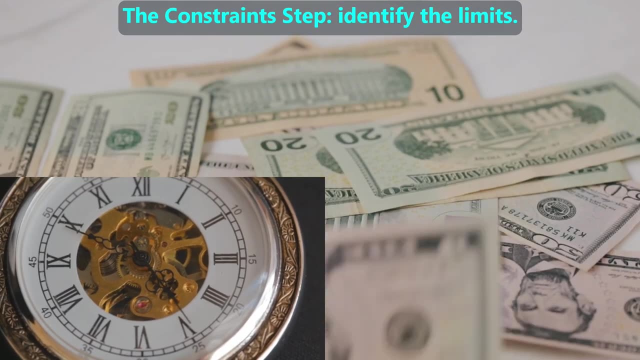 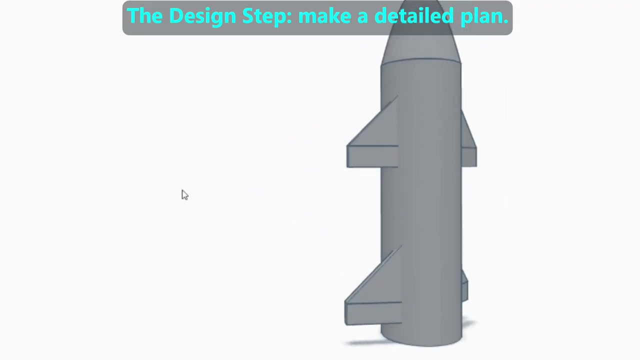 The engineers likely brainstormed many ideas for how to do this. This is the brainstorming step. Then the engineers likely identified constraints, which always includes money and time. This is the constraint step. Then they likely picked one of their brainstorm ideas that meets the constraints. 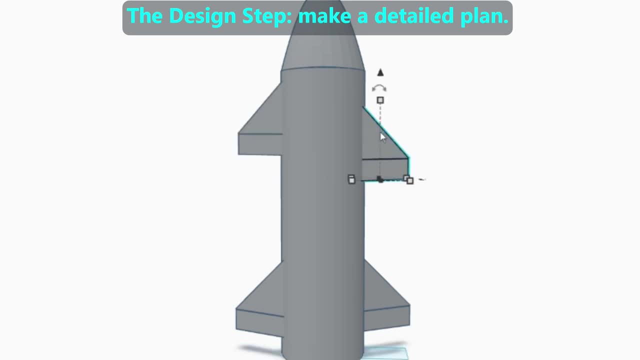 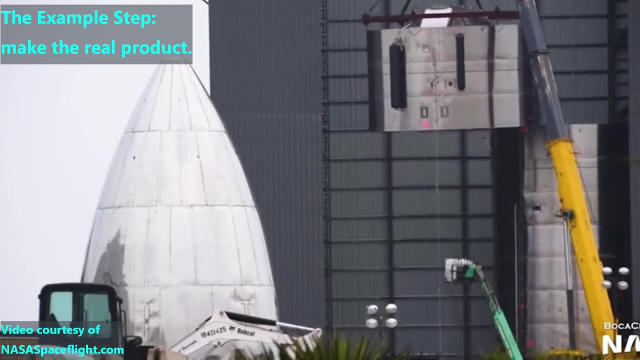 They made detailed designs using computers and small models using 3D printed parts. This is the design step. Then many people helped make a real Starship rocket out of real material and in its real size by following the details from the design step. 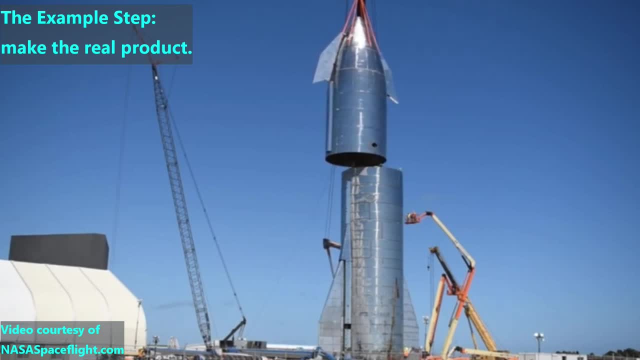 This is the example step. Unlike the prior scenario in which Angie's team made a museum, that is one of a kind, there will be many Starships. This is the example step. The project is set in the Starship example products. Each example product is a prototype. 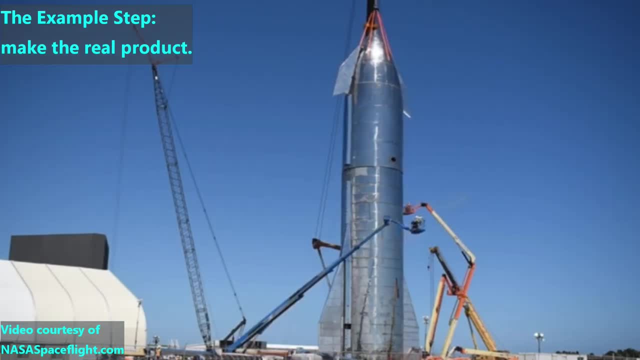 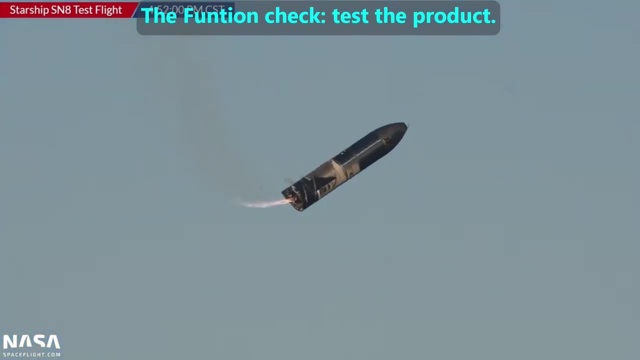 The purpose of a prototype is to test it during the function check so we know which design works. The next step is the function check. That means they test the example product, also known as a prototype, to see if it can launch and land. 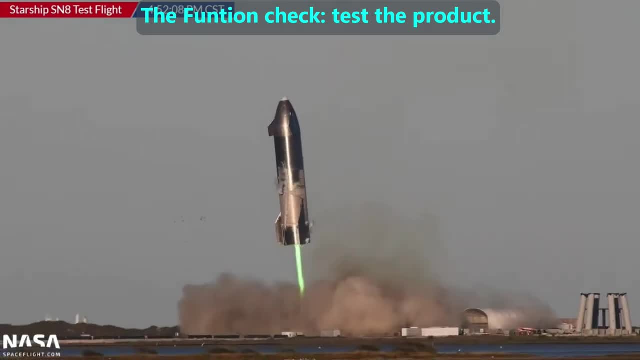 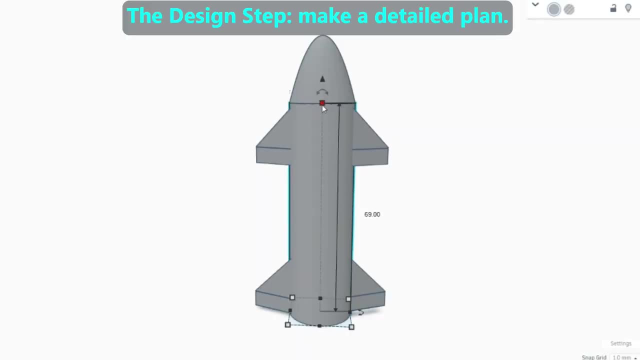 This is an actual video of the 8th prototype, which is called Starship, Serial Number 8.. Unfortunately, this prototype failed the function check. So the engineers went back to the drawing board, which means they returned to the design step, made some minor changes in the design, then built a new example product in real materials. 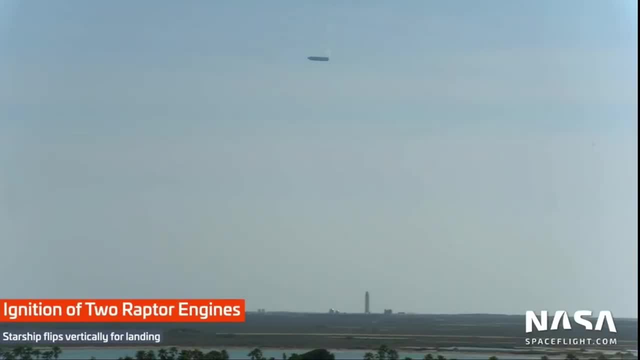 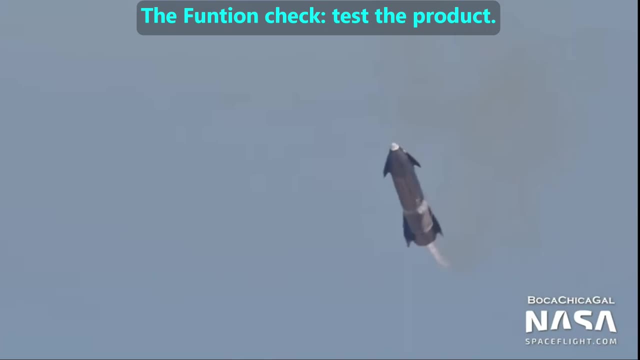 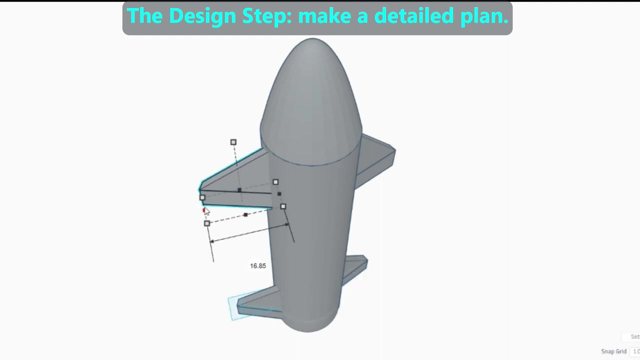 and in the real size. then did another function check. This is the ninth prototype, which is called Starship number 9.. Unfortunately it failed the function test Once again. the engineers went back to the drawing board, which means they returned to. 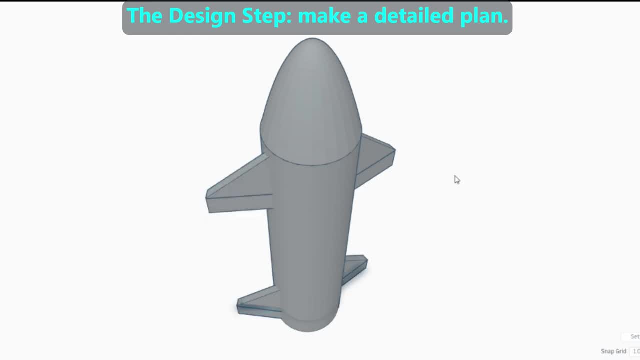 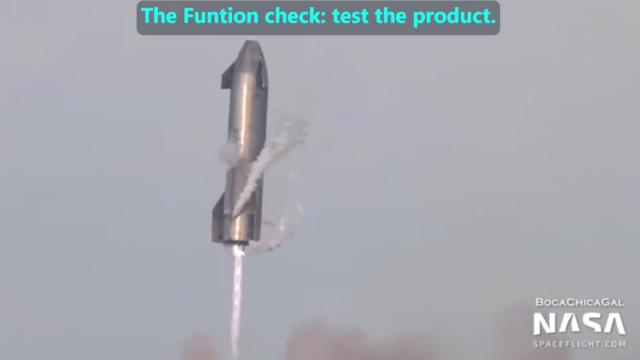 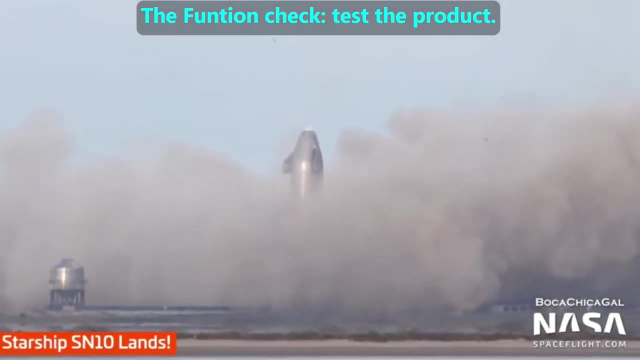 the design step, made some minor changes in the design, then built a new example product in real materials and in the real size, then did another function check. This is the tenth prototype, which is called Starship number 10.. This time it passed. 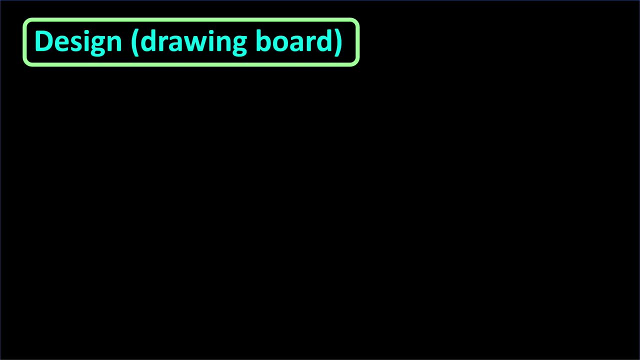 The fourth step in the engineering design process is to design. In this step the engineers make drawing. Some do this using a drawing board. The fifth step of the engineering design process is to make an example product. This is made of real materials and is the real size. 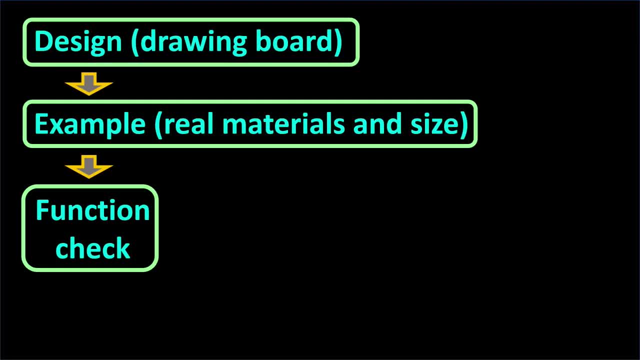 The sixth step of the engineering design process is to do a function check. That means to test the example product. If the example product passes the function check, then we're done with the engineering design process for this project. In this case, the tenth rocket prototype passed. 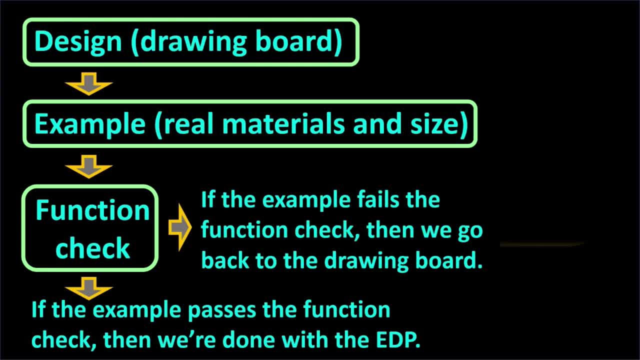 But if the example product fails the function check, then the engineers go back to the drawing board, which means to make some design changes, Make another example product and test it again. This is what the SpaceX engineers did after the eighth and ninth Starship prototype rockets. 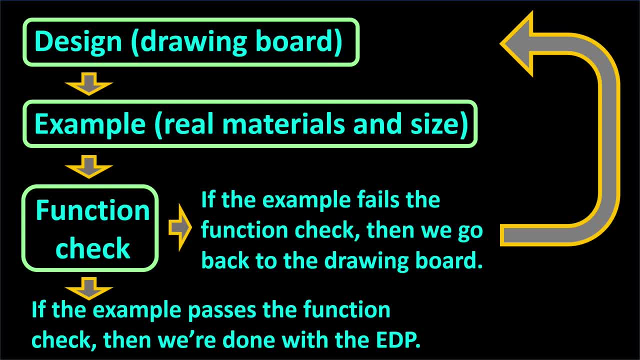 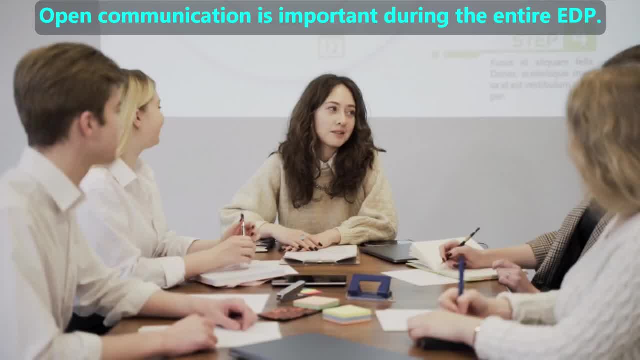 crashed instead of landing properly. This cycle of repeating steps is where the expression back to the drawing board comes from: whenever people have a project fail. A good design team has a leader that welcomes every member to space. This is what the SpaceX engineers did after the eighth and ninth Starship prototype rockets. 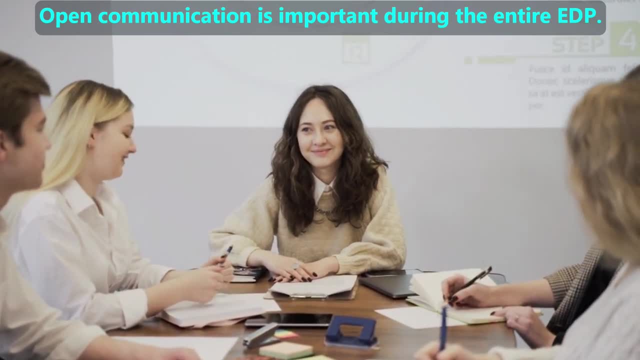 crashed instead of landing properly. This cycle of repeating steps is where the expression back to the drawing board comes from. whenever people have a project fail. If it fails, their team member should speak up if they or she has a concern or a constructive. 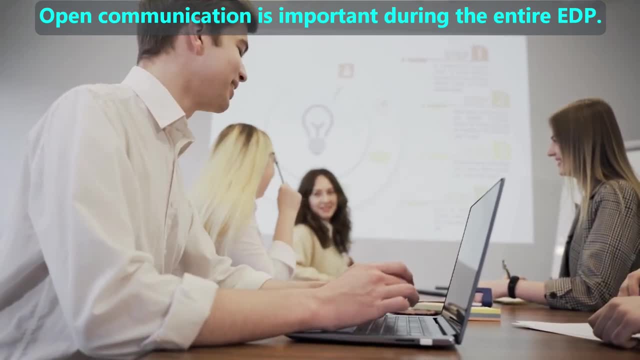 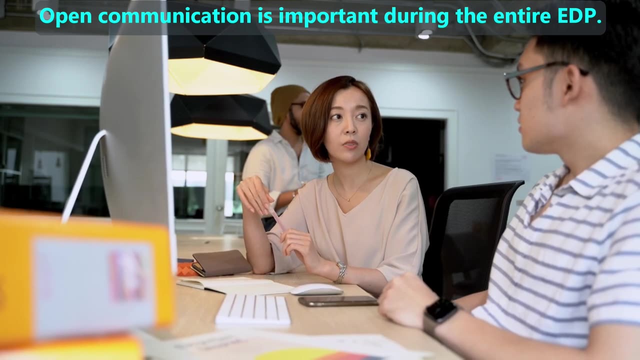 criticism. It is far less expensive to make a design change early on than to have recall a product later due to a part that is flawed. Plus, we all want to ensure the products we make are safe, So it would be terrible to notice a flaw and not say anything. and then somebody gets.